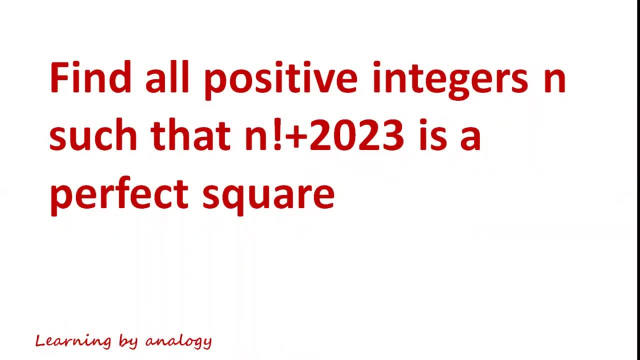 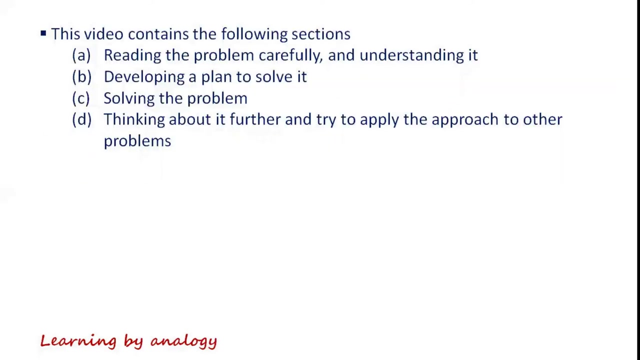 Find all positive integers n, such that n factorial plus 2023 is a perfect square. This video contains the following sections: Reading the problem carefully and understanding it. Developing a plan to solve it. Solving the problem. Thinking about it further and try to apply the approach to other problems. 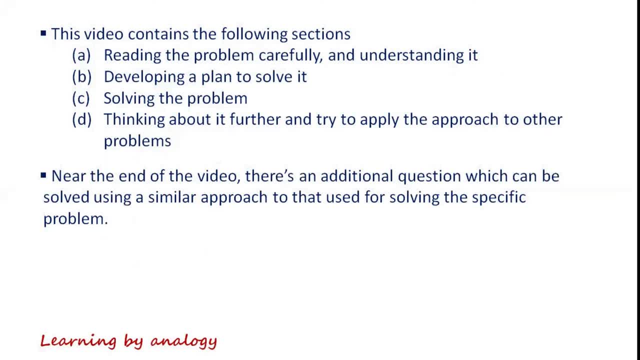 Near the end of the video, there's an additional question which can be solved using a similar approach to that used for solving the specific problem. If you find these helpful, please subscribe to the channel for notification of new videos by pressing the video watermark in the right hand corner of the video player. 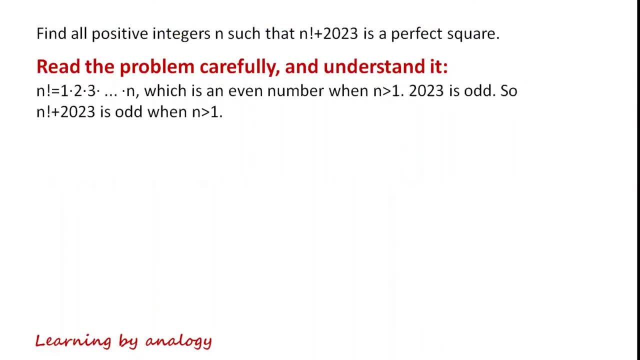 n? factorial equals one times two times three. Please subscribe to the channel for notifications of new videos. So this is a very simple problem. This is a very simple problem. The following equation is an example for solving the problem, So I'll show you how. 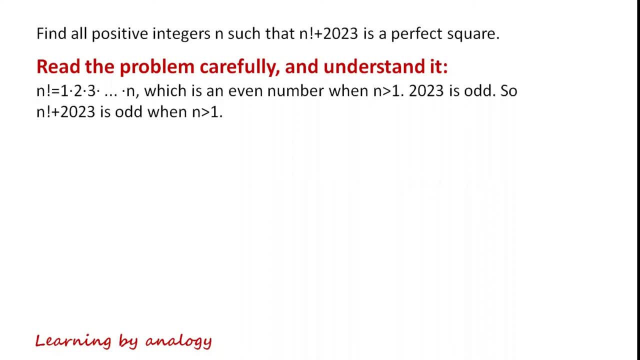 So I'll say n factorial times. so on times n and 23 is odd when n is greater than 1.. It seems a perfect way to determine if a number is a perfect square, apart from verification, doesn't exist. However, to prove a number isn't a perfect square might be relatively. 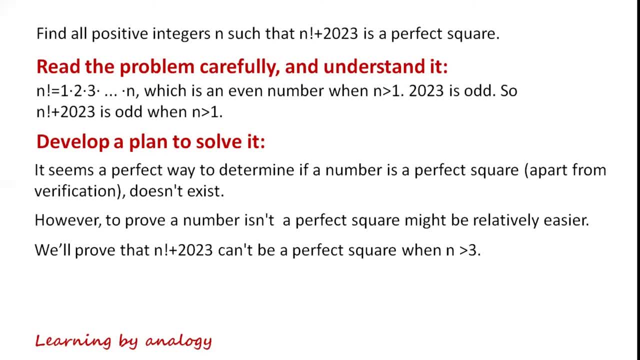 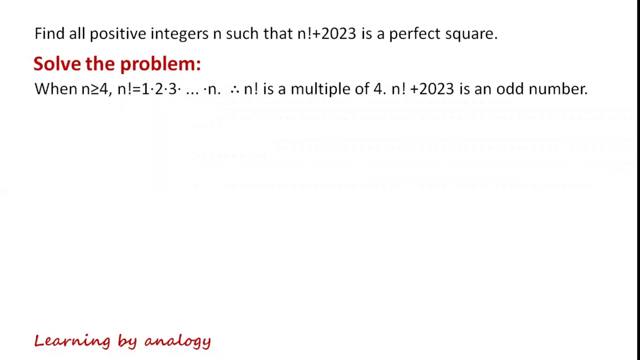 easier. We'll prove that n factorial plus two thousand and twenty-three comes out to be a perfect square. When n is greater than three, then check specific cases when n is less than or equal to three. When n is greater than or equal to four, n factorial equals three. 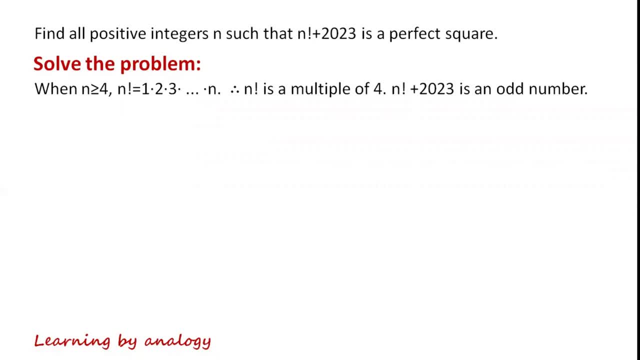 It's a multiple of four And factorial plus two thousand and twenty-three is an odd number because 2023 is congruent to 3 mod 4.. So n factorial plus 2023 is congruent to 3 mod 4.. 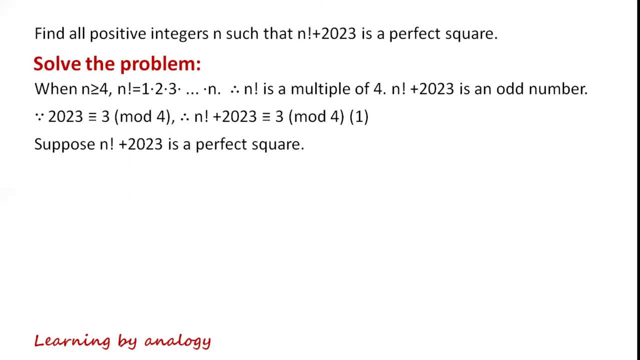 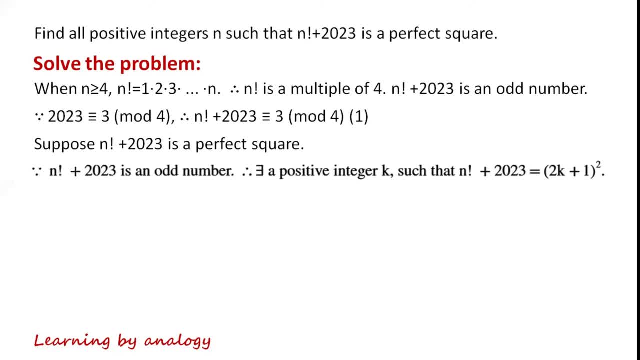 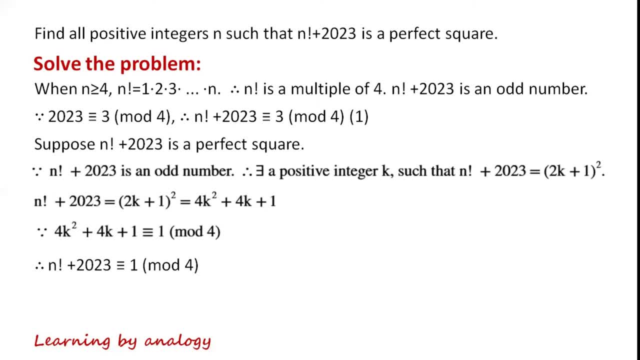 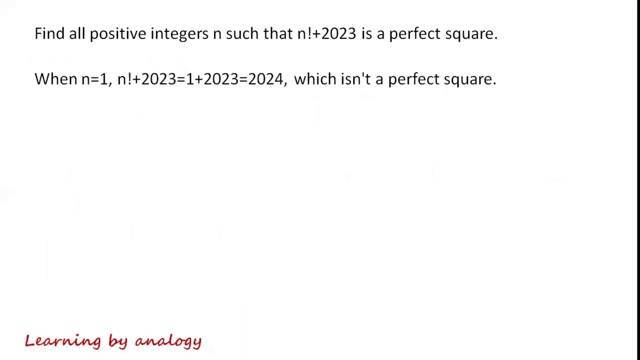 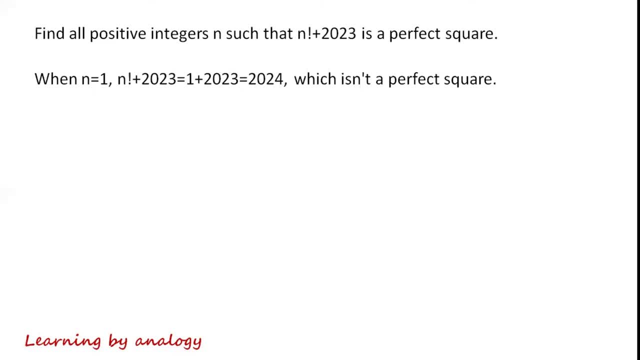 So? n factorial plus 2023 is congruent to 1 mod 4.. So n factorial plus 2023 is congruent to 1 mod 4.. equals 1 plus 2023, which is equal to 2024, which isn't a perfect square when n equals. 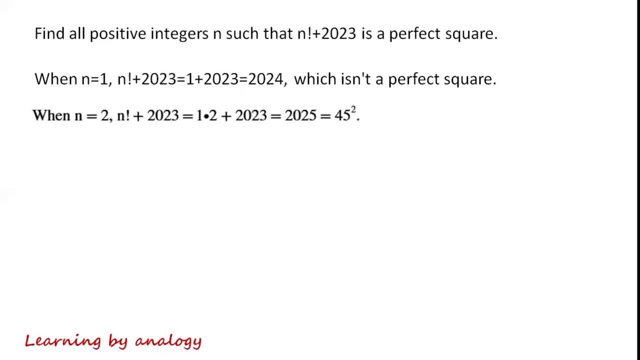 2, n factorial plus 2023 equals 1 times 2 plus 2023,, which is equal to 2025,, which is equal to 45 squared When n equals 3, n factorial plus 2023 equals 1 times 2 times 3 plus 2023,, which is equal. 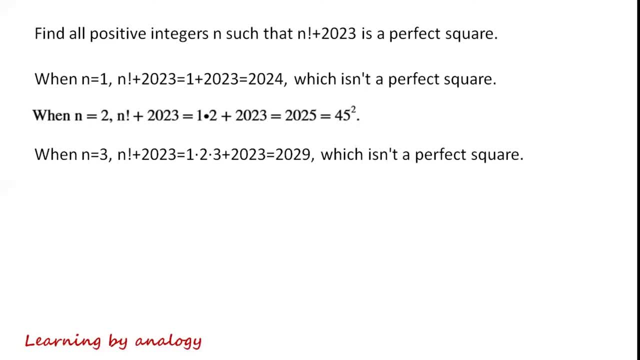 to 2029.. Which isn't a perfect square, because n factorial plus 2023 can't be a perfect square for n equals 1, n equals 3, for all n greater than or equal to 4.. So n factorial plus 2023 is a perfect square for n equals 2 only. 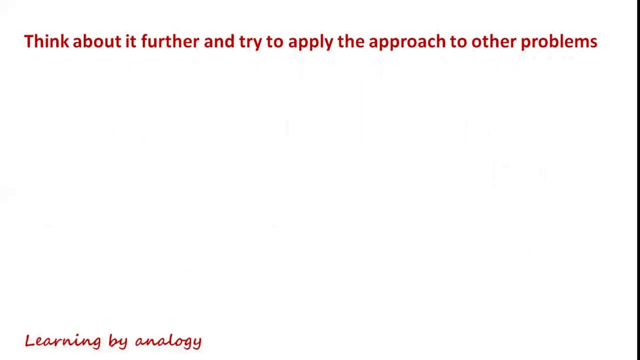 Think about the thought process for the previous question further and try to apply the approach to other problems Such as this. one Suppose that n is an even constant and n is in the set of natural numbers. That's proof that m squared n squared plus 9,999 can't be a perfect square.